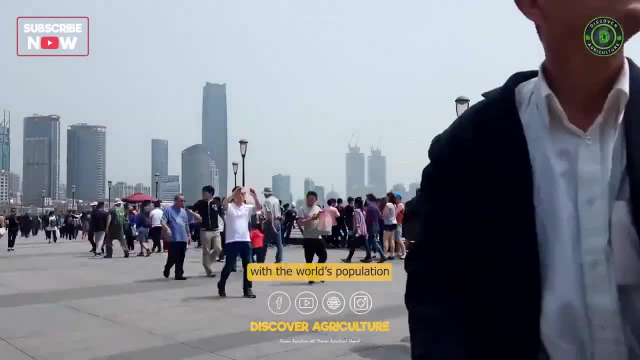 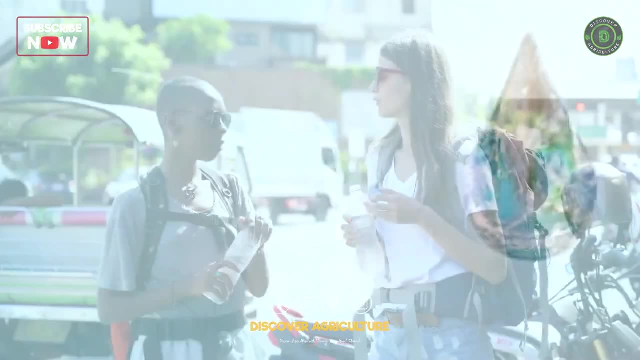 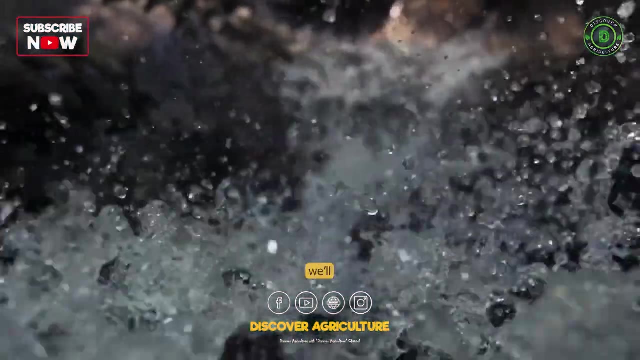 notifications on new videos. However, with the world's population increasing rapidly, the demand for water is increasing at an unprecedented rate. That's why it's important to manage our water resources effectively. In this video, we will be talking about an innovative solution: the Integrated Water. 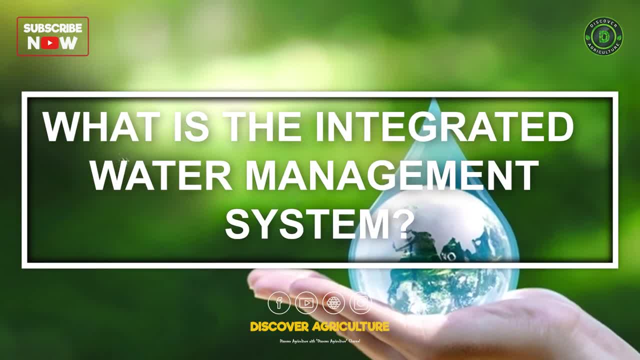 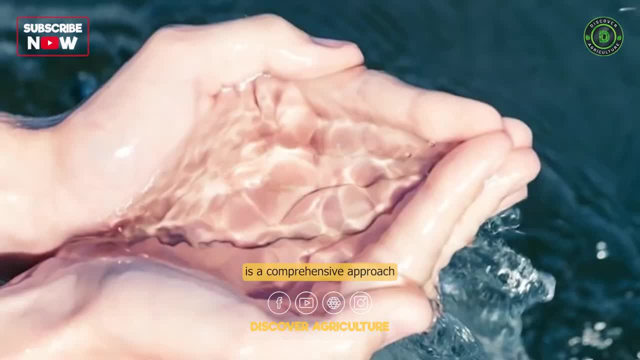 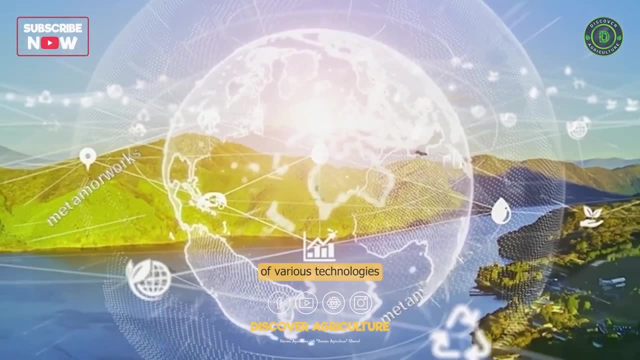 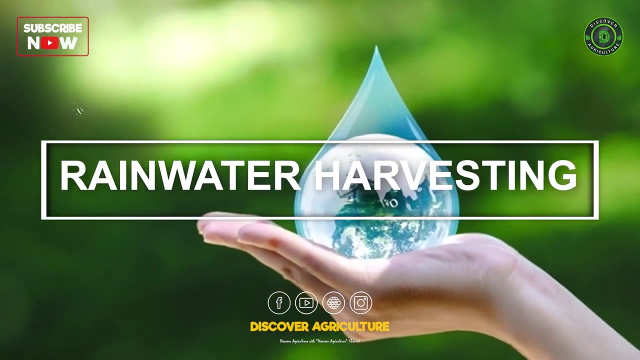 Management System. 1. What is the Integrated Water Management System? The Integrated Water Management System, or IWMS, is a comprehensive approach to managing water resources. It involves the integration of various technologies and strategies to ensure that water is used efficiently and effectively. 2. Rainwater Harvesting. 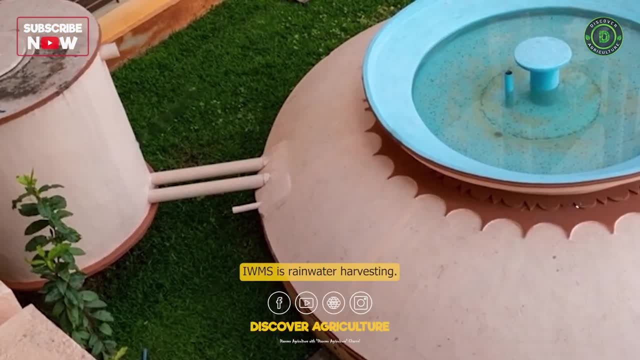 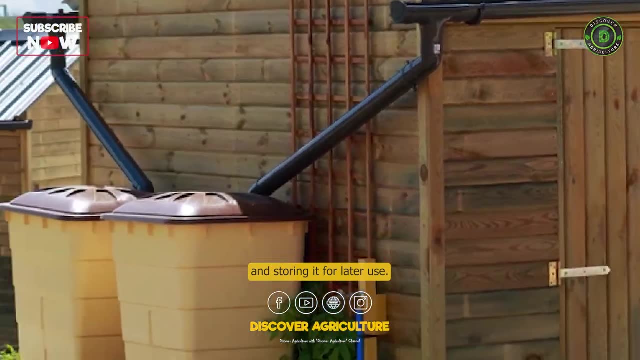 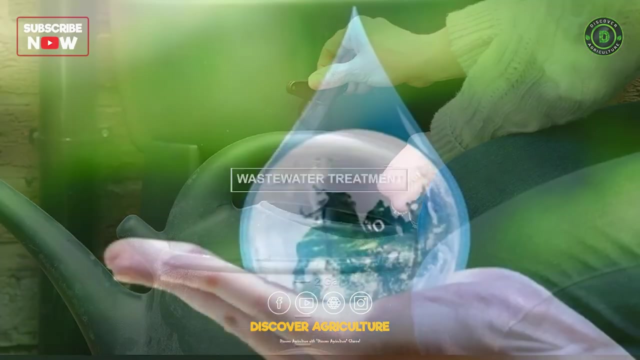 One of the key components of the IWMS is rainwater harvesting. This involves capturing rainwater and storing it for later use. This not only helps conserve water, but also helps reduce the demand for treated water. 3. Wastewater- Wastewater treatment. Another important component of the IWMS is 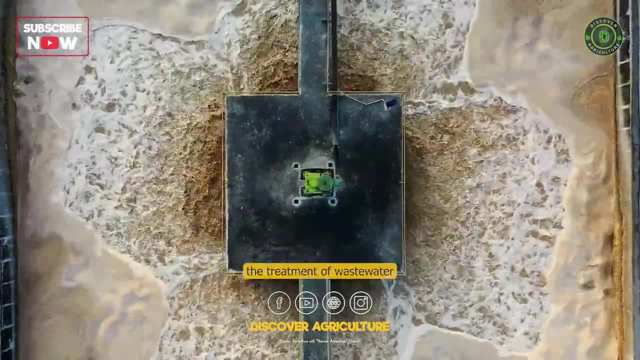 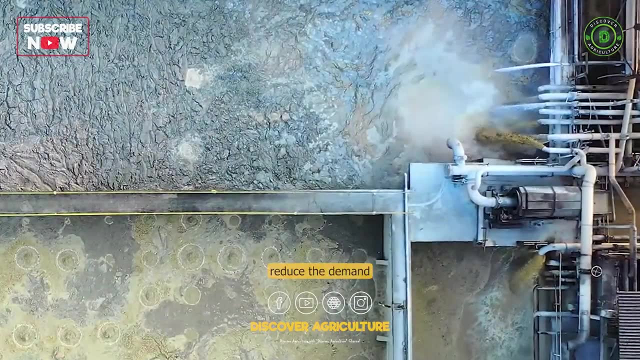 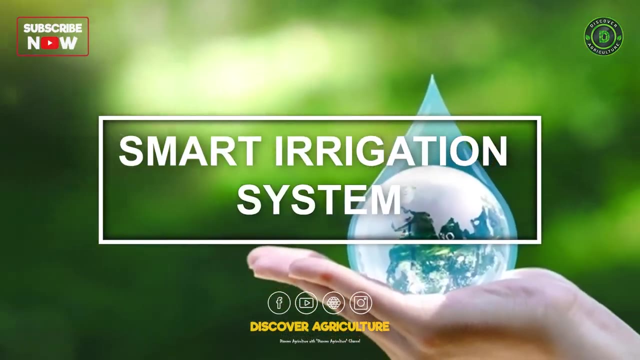 wastewater treatment. The system involves the treatment of wastewater to remove contaminants and make it safe for reuse. This helps reduce the demand for fresh water and also helps prevent pollution of our water bodies. 4. Smart Irrigation Systems. The IWMS also includes the use of smart irrigation systems. 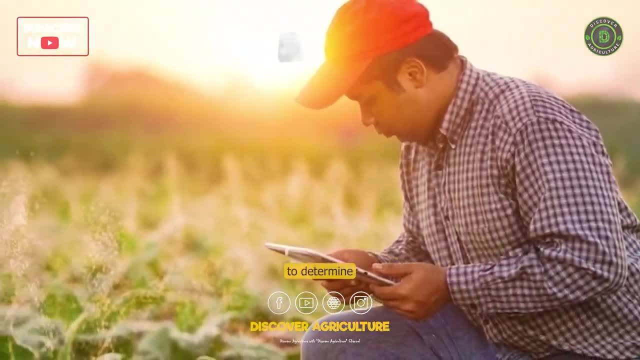 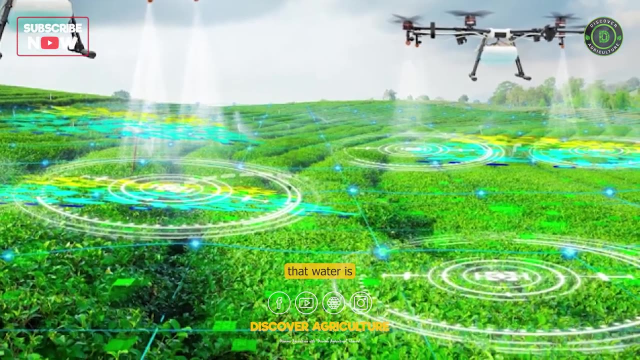 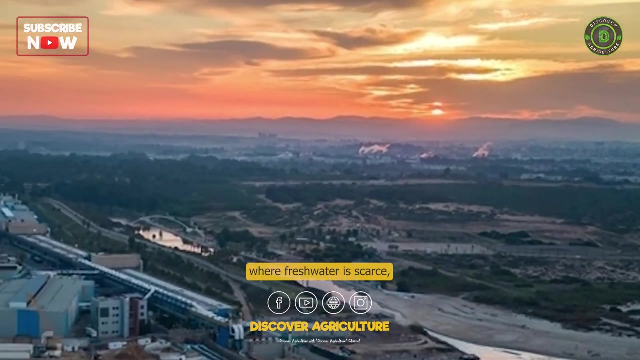 These systems use sensors and weather data to determine the optimal amount of water needed for plants. This helps prevent overwatering and ensures that water is used efficiently. 5. Weed Desalination Plants In areas where fresh water is scarce. the IWMS also includes the use of desalination plants. 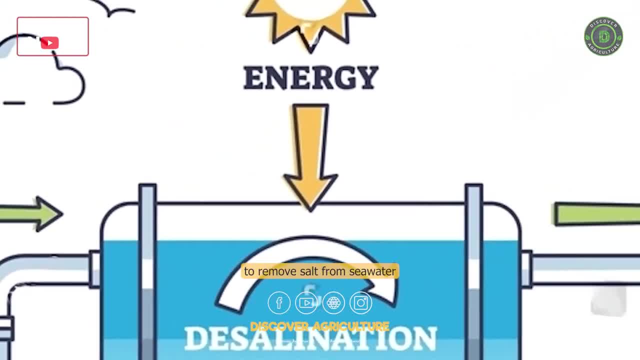 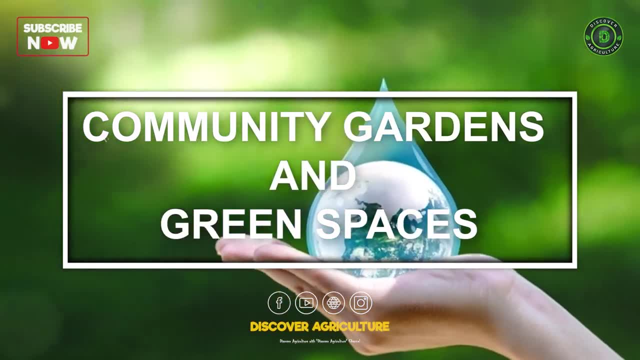 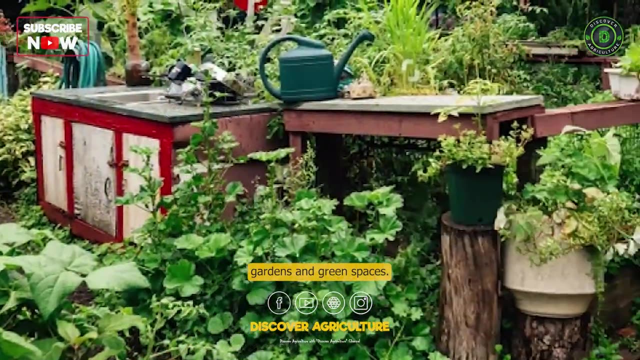 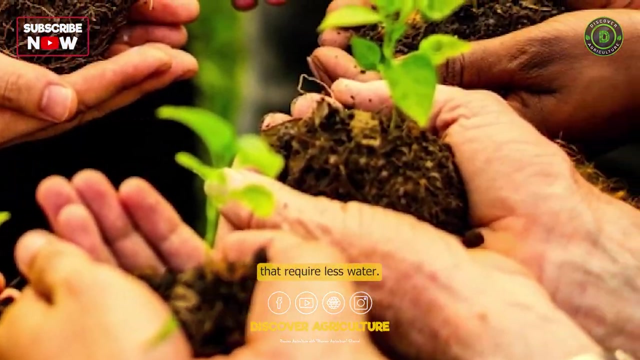 These plants use advanced technology to remove salt from seawater and make it safe for drinking, drinking and other uses. 6. Community Gardens and Green Spaces. Finally, the IWMS encourages the use of community gardens and green spaces. These spaces help reduce the demand for water by promoting the use of native plants that require.